Hello, I am your teacher Lara and today I'll teach you about adding three or more digits and here we go. Start number one, 1235 plus 622 so alignment is very important so that you can arrive or you can get the right or the correct answer. So 5 plus 0 is equals to 5. 3 plus 2 is equals to 5. 2 plus 6 is equals to 8. And 1 since there is no value here so you just dropped down the 1. So the answer here is 1855. So now we're done here. 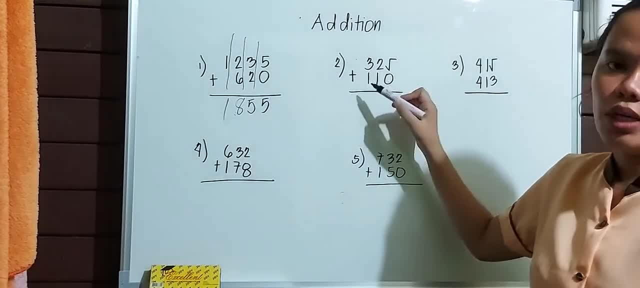 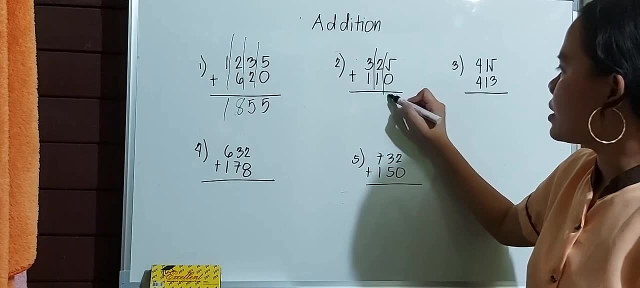 two three hundred twenty five plus one hundred ten so five align align so five plus zero is equals to five two plus one is equals to three three plus one is equals to four 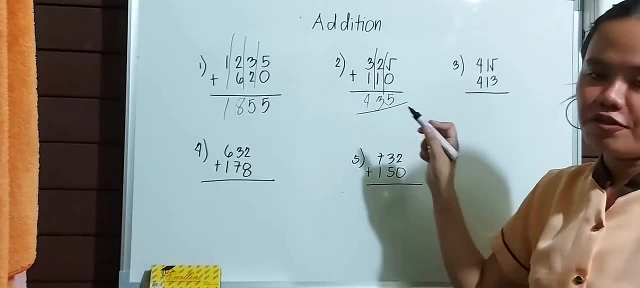 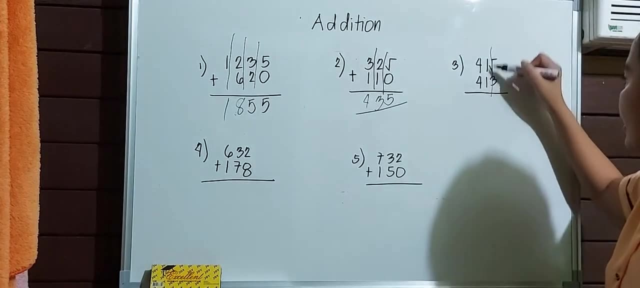 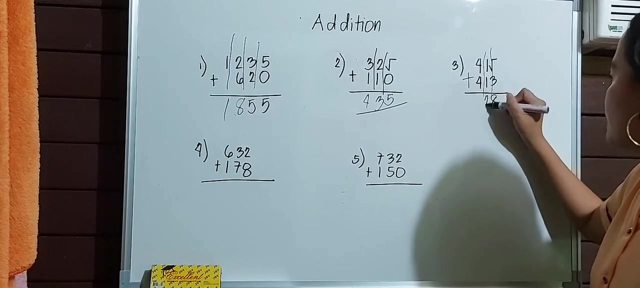 so the answer here is 435 the next one is 415 plus 403 so so align align so five plus three is equals to eight one plus one is equals to two plus 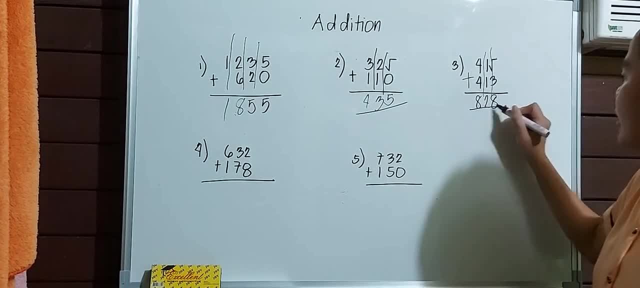 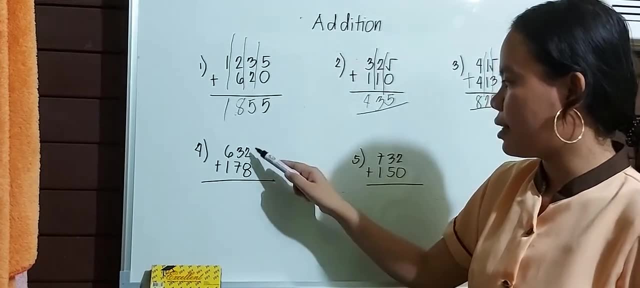 four plus four is equals to eight so the answer here is 820. so the next one is 632 plus 178 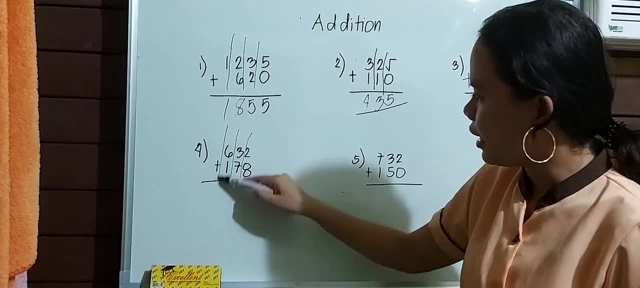 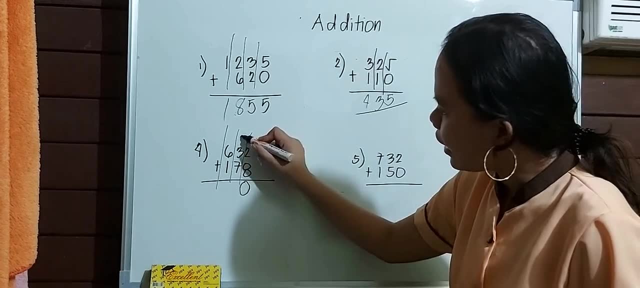 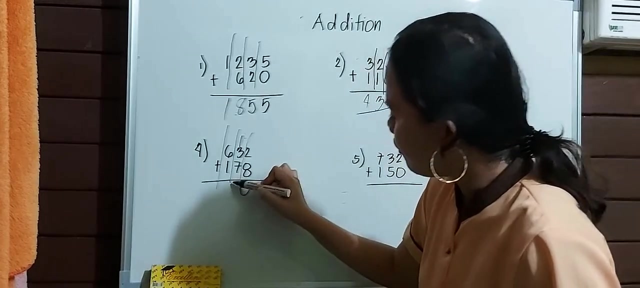 two align align again align so two plus eight is equals to ten so bring down zero and add one so one plus three is four plus seven is 11 so bring them one add one here so one plus 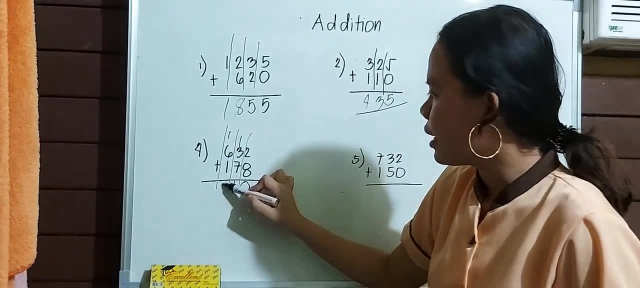 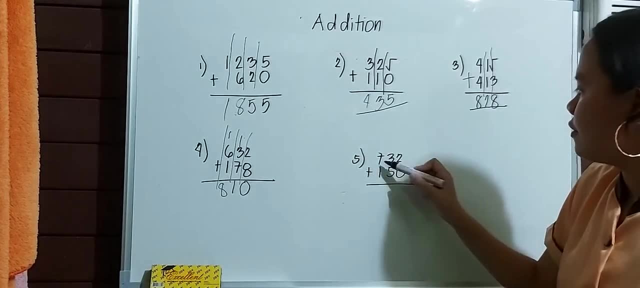 six is seven plus one is eight so the answer here is 810. so the last one is 732 plus 150. 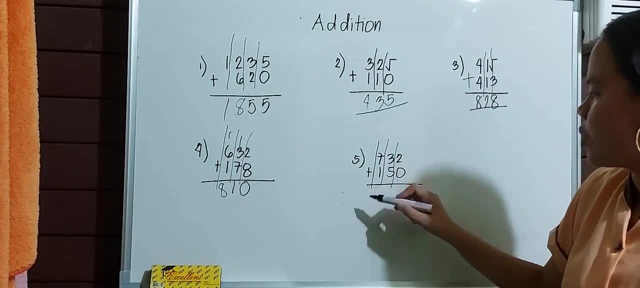 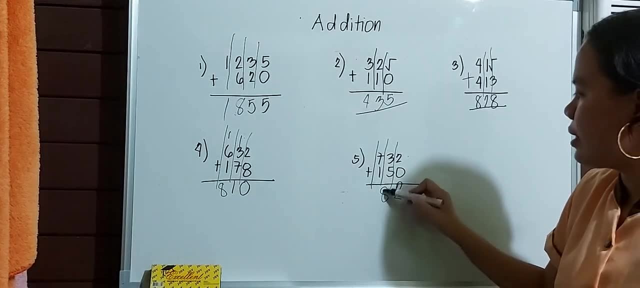 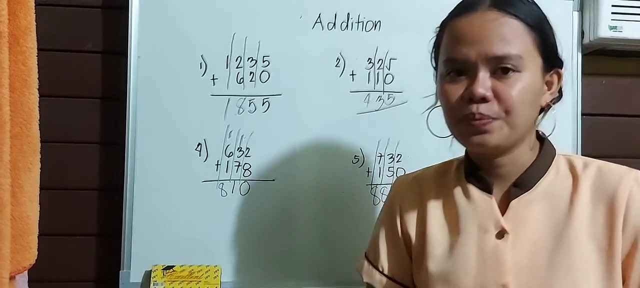 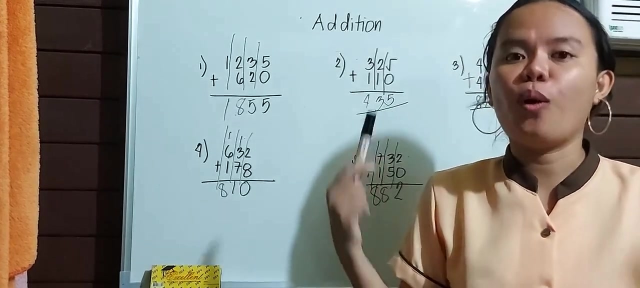 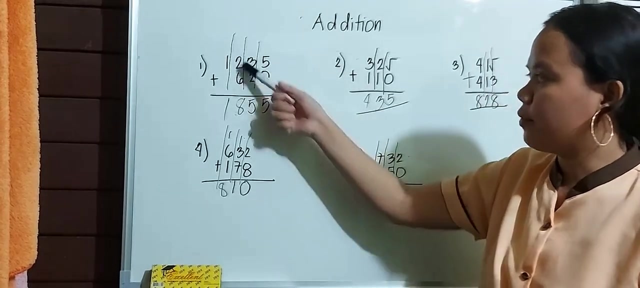 so align align again and this one so two plus zero is two three plus five is eight seven plus one is equals to eight so the answer here is 882. so addition and counting is very important so that if you know how to count make sure you know how to add and of course always remember that when you were adding alignment of the place above you is very important so that you can arrive with your right answer. And that's all for today. Thank you! 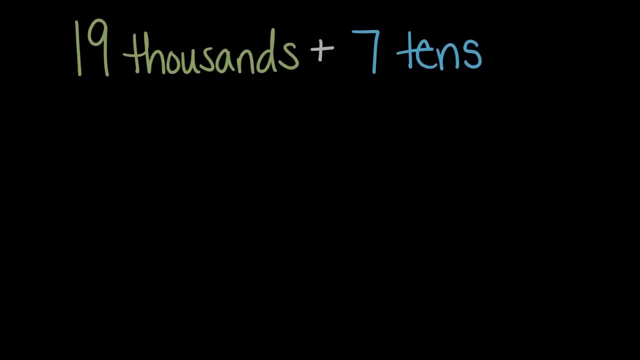 What is 19,000s plus seven 10s? First, let's think about what are 19,000s and what are seven 10s, and then from there we can add them.